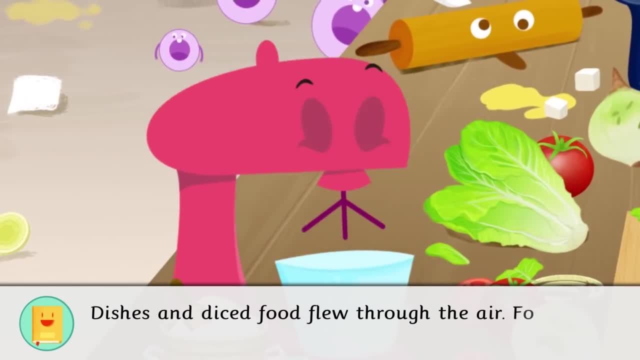 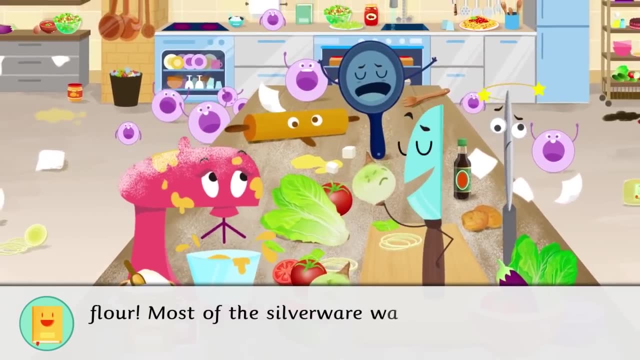 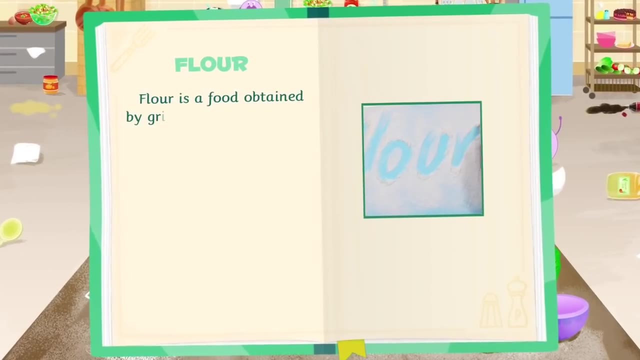 Dishes and diced food flew through the air. Food processor: processed and processed. It was snowing. flour- Most of the silverware was crying from cut onions. Flour is a food obtained by grinding up grains like wheat, rye or oats. 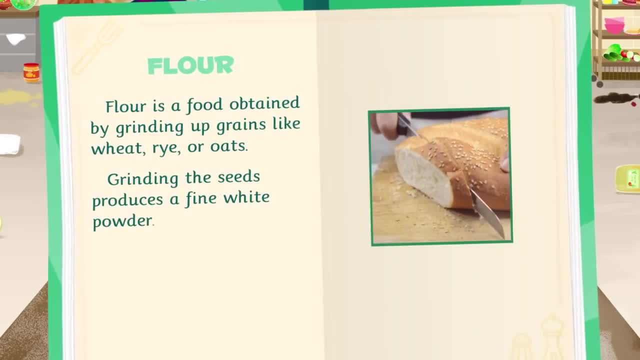 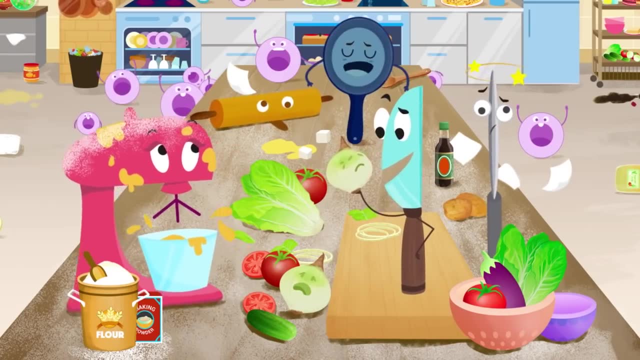 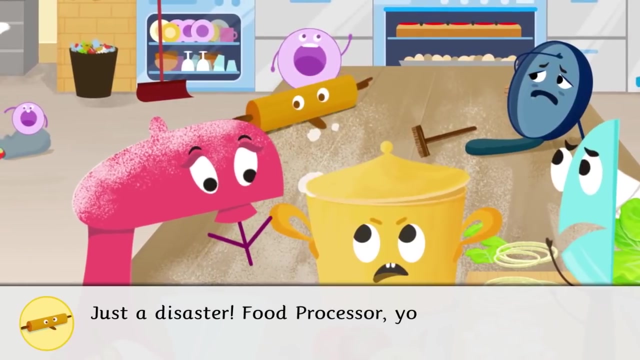 Grinding the seeds produces a fine white powder. Wheat is the main ingredient in bread. The flour is the main ingredient in bread. Just a disaster, Food processor. you've got everything covered in flour. Sam can't eat any gluten, remember. 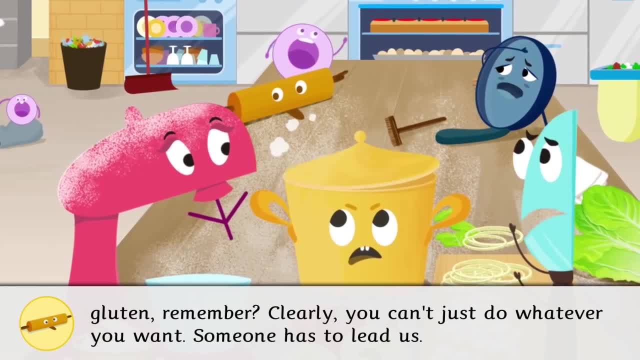 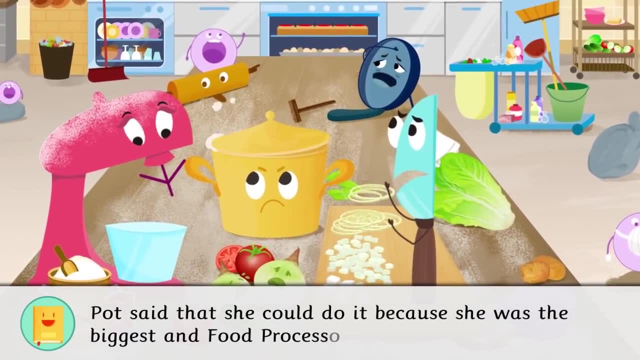 Clearly you can't just do whatever you want. Someone has to lead us. Pot said that she could do it because she was the biggest, And food processor said she should do it because she was the biggest. And food processor said she should do it because she was the biggest. 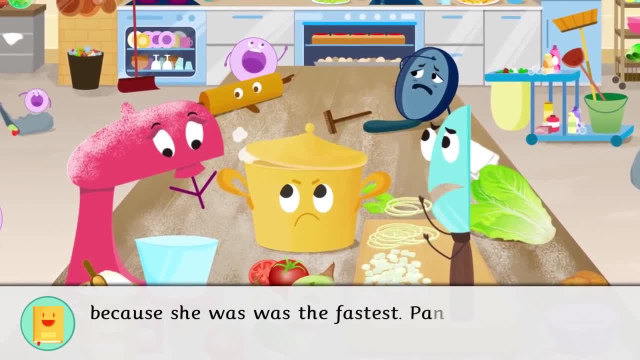 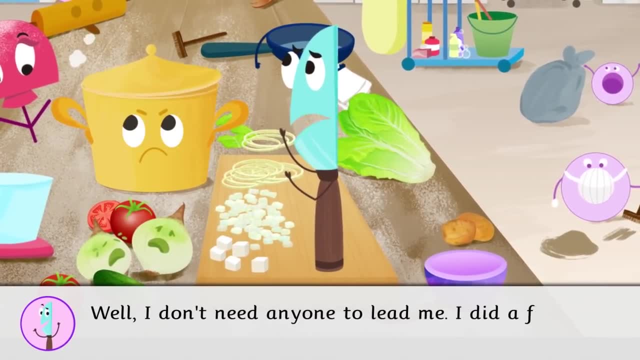 And food processor said she should do it because she was the biggest Pan, just wanted to doze on the burner. Well, I don't need anyone to lead me. I did a fine job. Apparently, I'm the only one. Maybe I should go to another kitchen. 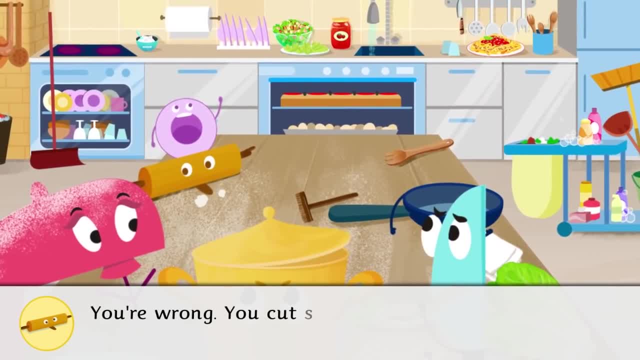 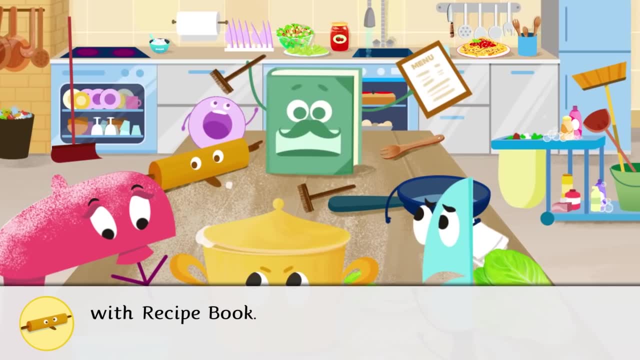 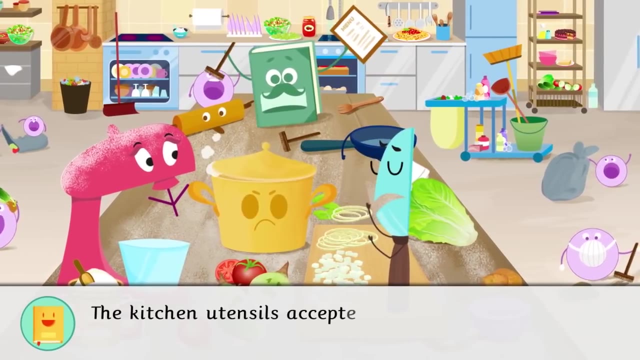 You're wrong. You cut so much onion up and everyone ended up crying. You cut so much onion up and everyone ended up crying. I think we should consult with recipe book. I think we should consult with recipe book. knows the ingredients we need and steps to take. The kitchen utensils accepted his proposal. 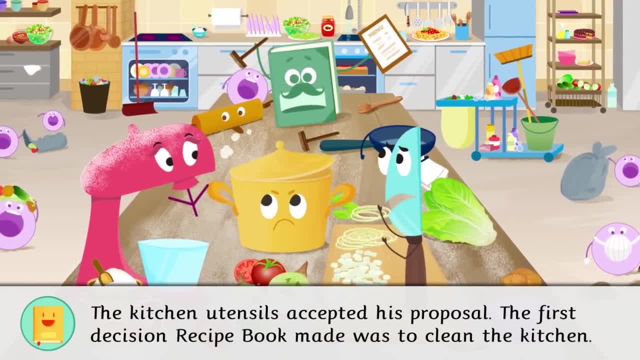 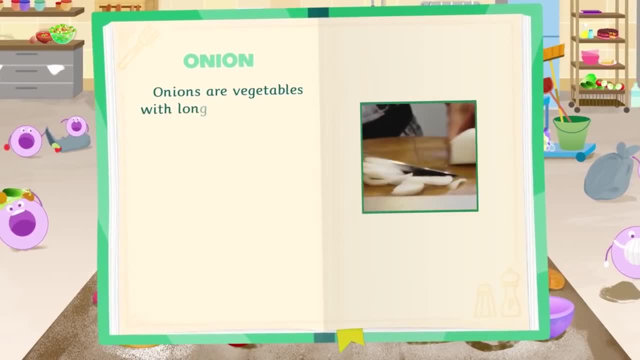 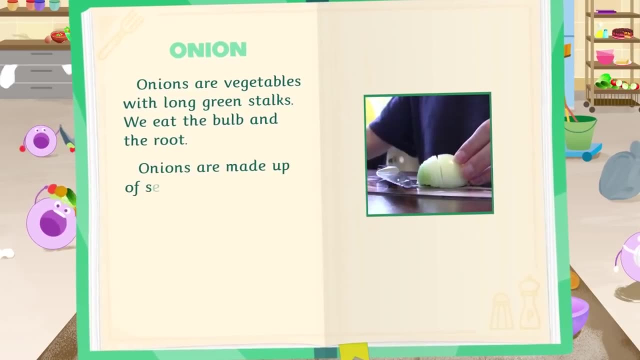 The first decision Recipe Book made was to clean the kitchen. Then he got everyone cooking. Onions are vegetables with long green stalks. We eat the bulb and the root. Onions are made up of several layers. When you cut open an onion, 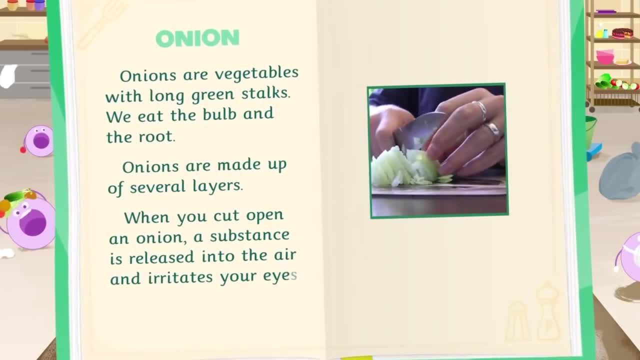 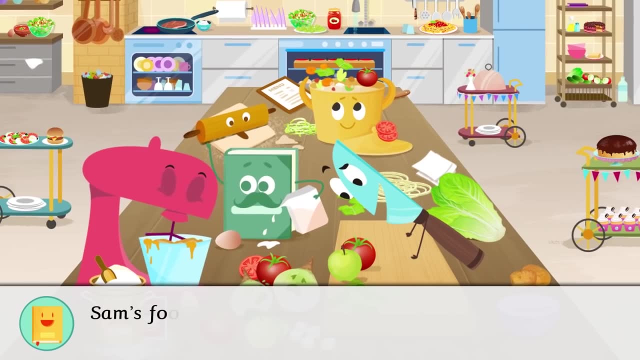 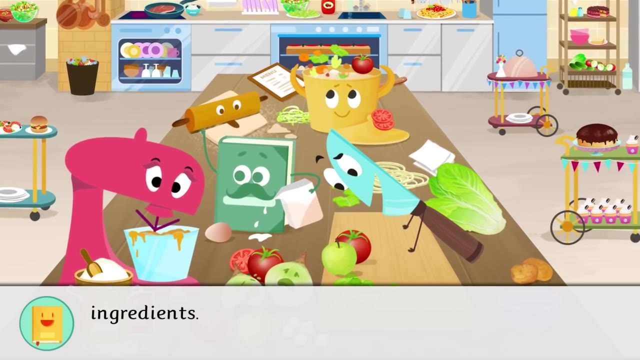 a substance is released into the air and irritates your eyes and nose. Sam's food was important and they started with his meal Recipe Book, sent them to look for the right ingredients, Then he told Knife to cut up the lettuce, tomato and apples for the salad. 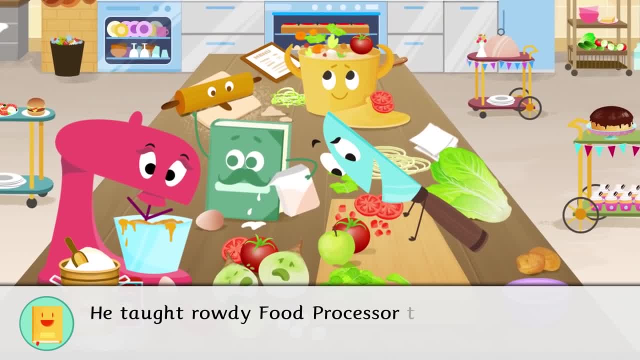 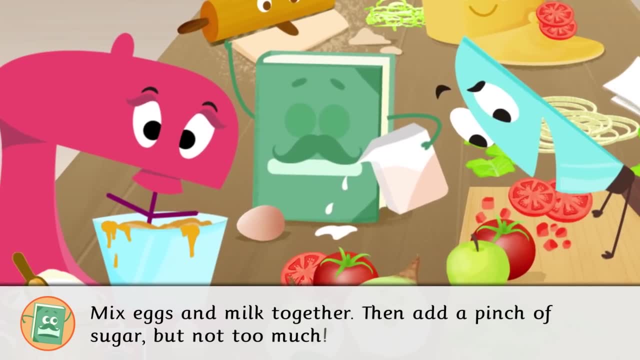 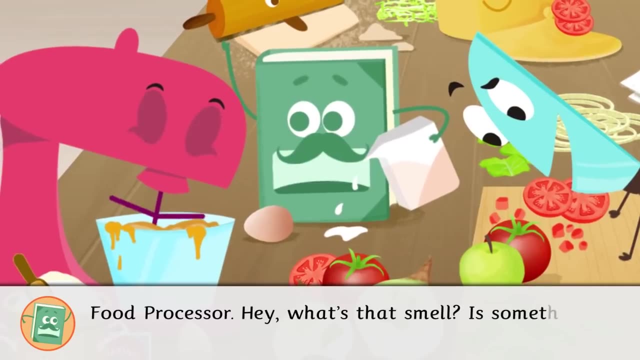 That was healthy. He taught Rowdy Food Processor to make flan, Mixed eggs and milk together, Then add a pinch of sugar, but not too much. Steady as she goes, Food Processor. Hey, what's that smell? Is something burning Pan? the steak is going to burn. Flip it over. 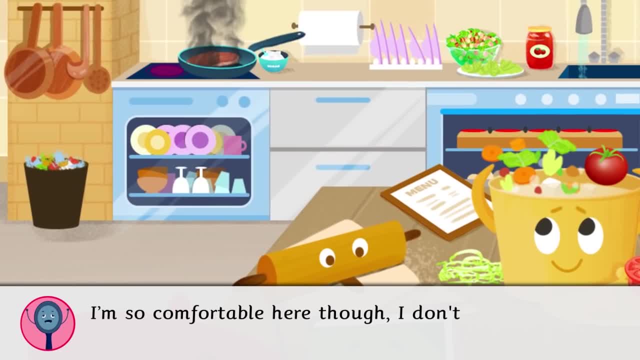 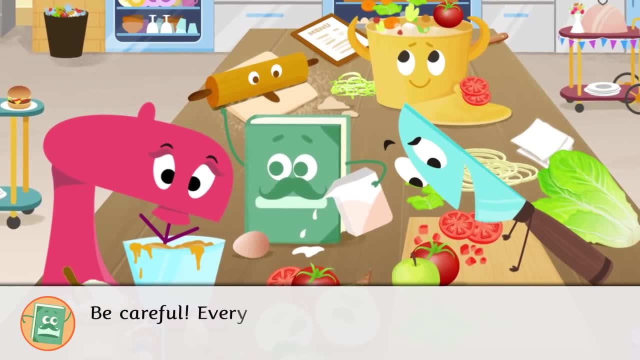 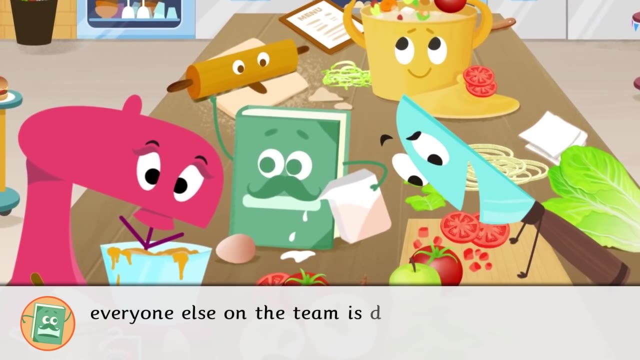 I'm so comfortable here though I don't want to move. Can I do it tomorrow? Be careful: Everyone else's work depends on yours. If one person makes a mistake, it will ruin what everyone else on the team is doing. 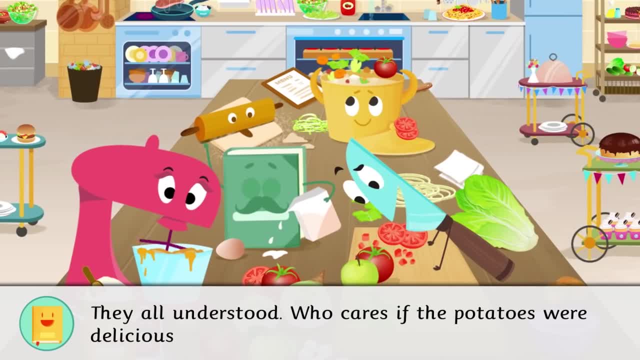 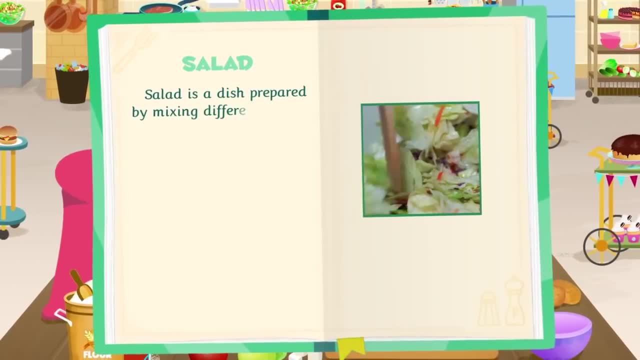 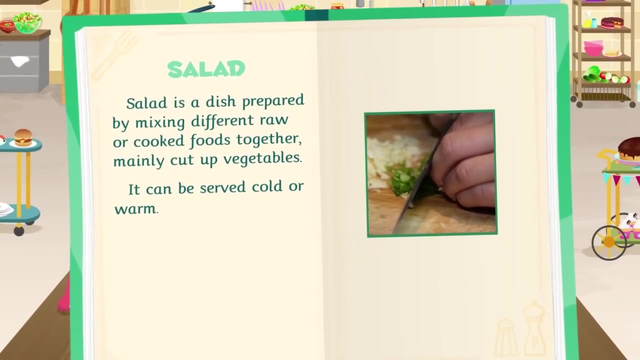 They all understood Who cares if the potatoes were delicious, if the steak was burnt. Salad is a dish prepared by mixing different raw or cooked foods together, Mainly cut up vegetables. It can be served cold or warm. You can make vegetable pasta. 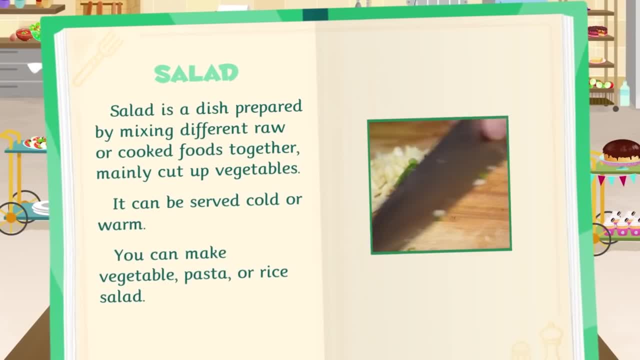 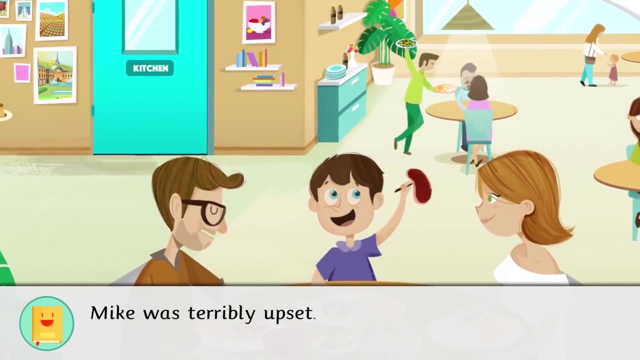 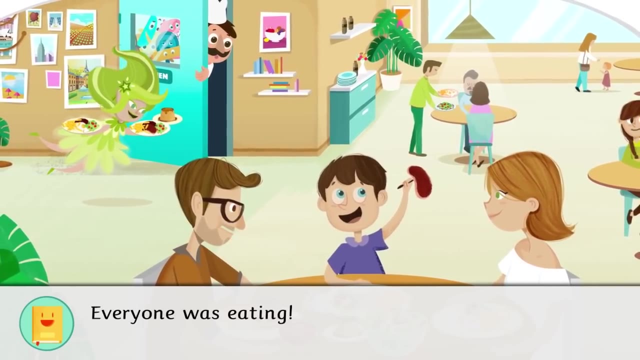 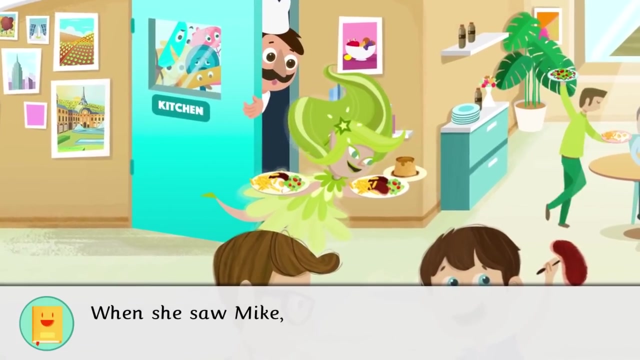 or rice salad. Mike was terribly upset. When he felt better he went to the restaurant's dining room to supervise Everyone was eating. The fairy godmother bustled from table to table serving guests and clearing plates. When she saw Mike, she winked at him. 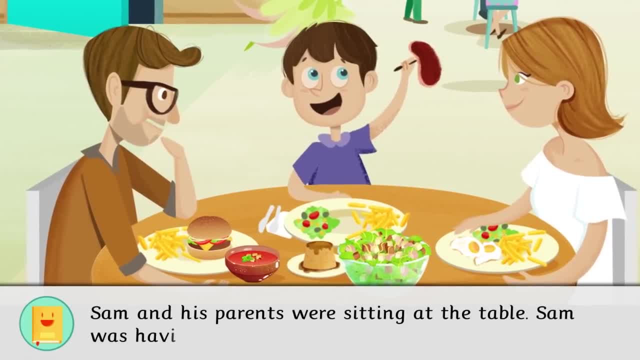 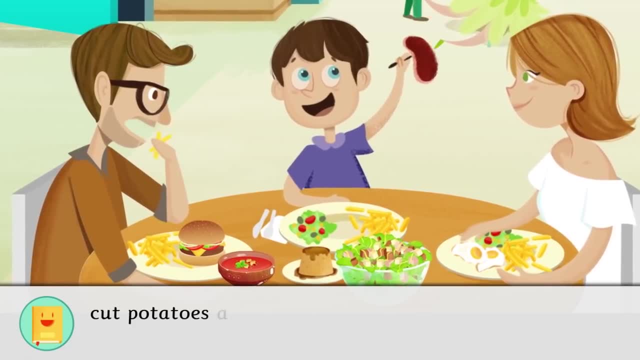 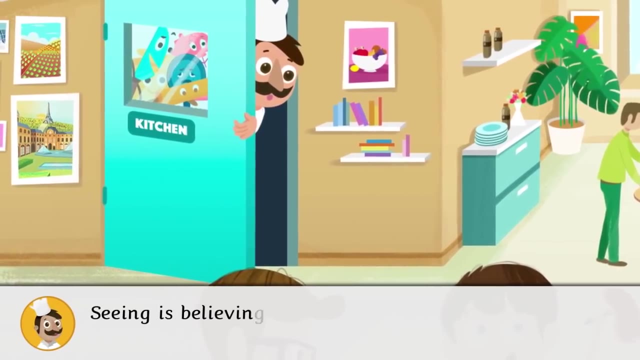 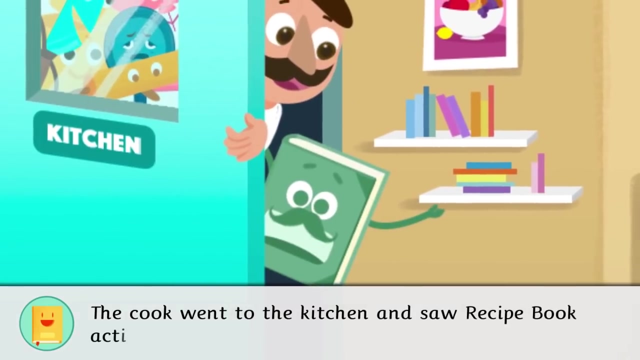 Sam and his parents were sitting at the table. Sam was having an absolutely fantastic meal: Steak, salad, cut potatoes and flan. It was just as he imagined it would be. Seeing is believing, but how did you do it? The cook went to the kitchen and saw a recipe book, acting as chef. 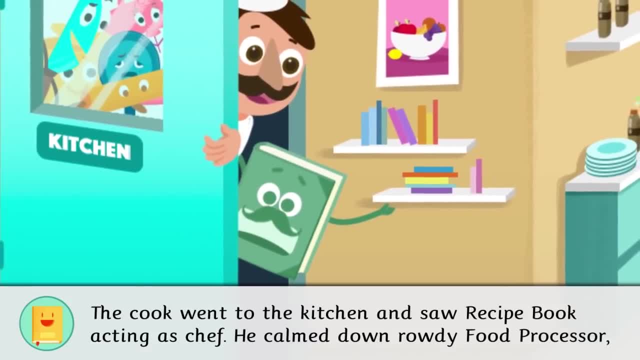 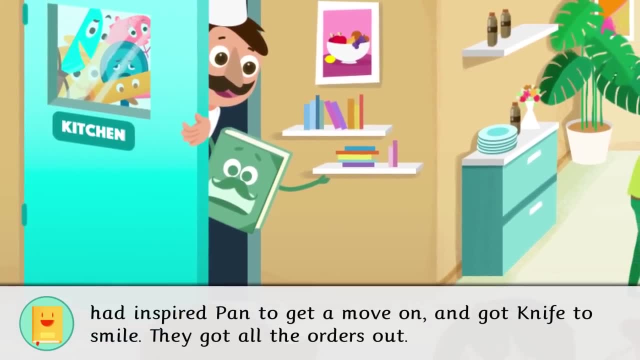 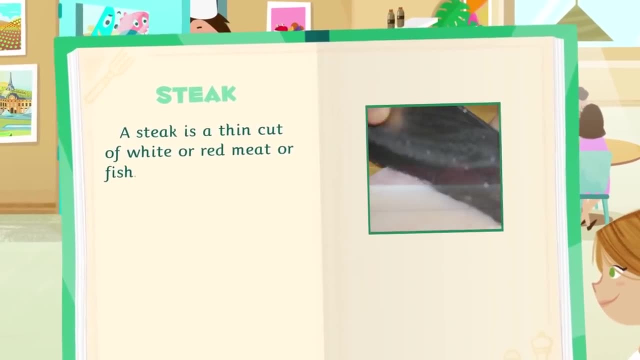 He calmed down rowdy food processor had inspired pan to get a move on and got knife to smile. They got all the orders out. A steak is a thin cut of white or red meat or fish. It's usually fried or breaded. 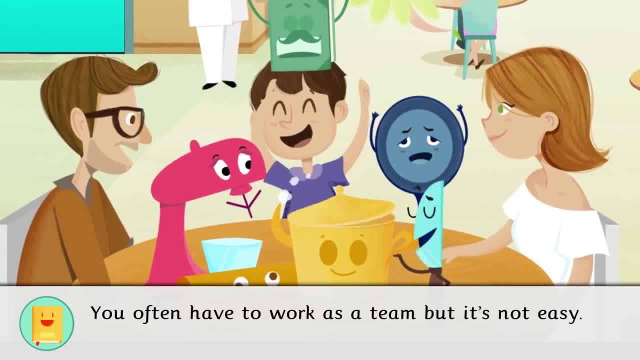 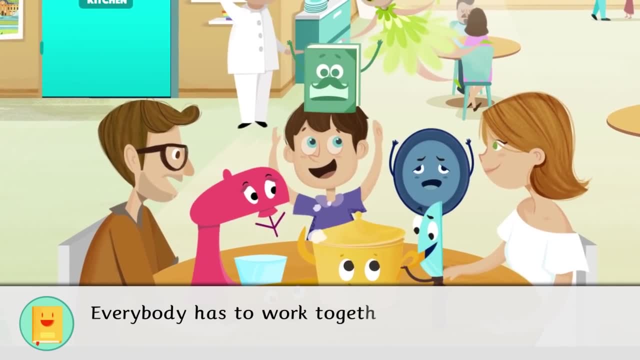 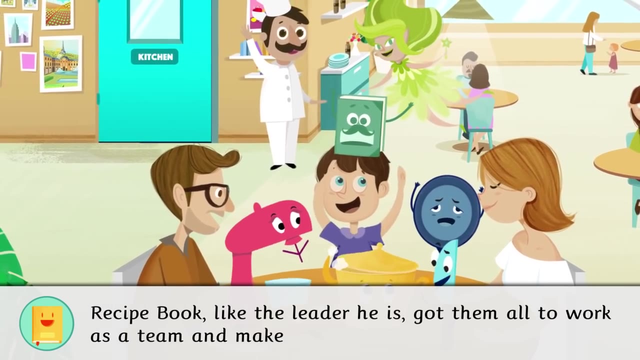 You often have to work as a team, but it's not easy. Everybody is special and has their own personality. Everybody has to work together. Recipe book. like the leader, he is got them all to work as a team and make a healthy meal. Yeah, Boijy Gh messaging sina a esta empresa. I do, to tell their story and reach their goal. 硫酸nt Drooling DistBTW, Because it's tough work. Where's mom Money? I know. Money.